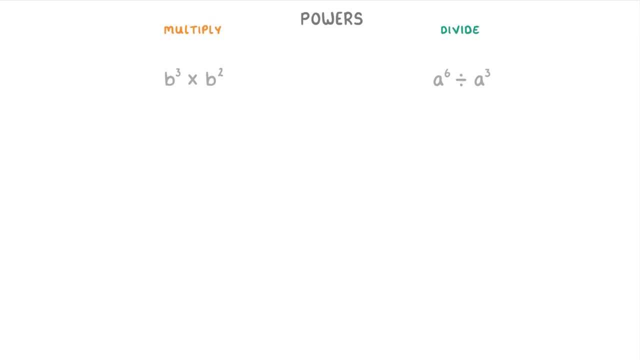 this topic is to think about what the powers really mean. If we start with this multiplication, one b cubed just means b times b times b, because the power of three means that we have three b's being multiplied together, Meanwhile b squared just means b times. 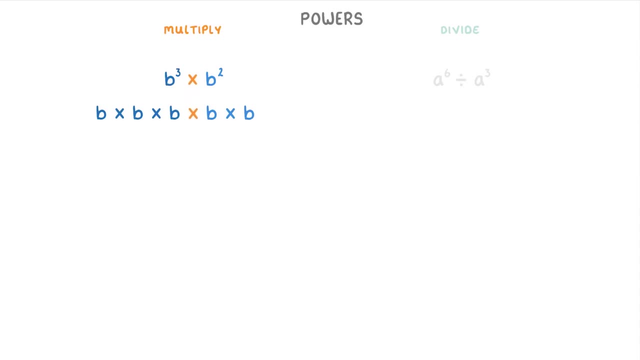 b, And so if we multiply these two terms together, we're just going to have five b's being multiplied together, which is the same thing as b to the power of five, So that's our answer. Instead of writing all of this out every time, though, the shortcut is to just add together the 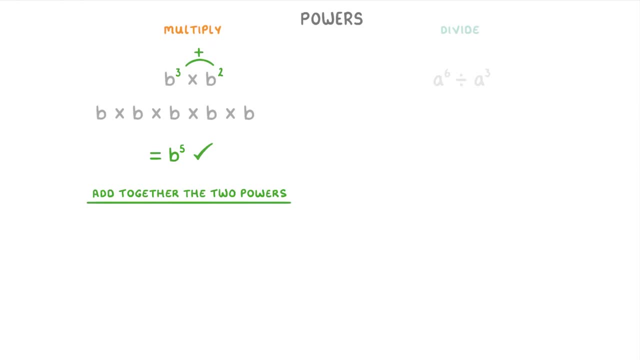 two powers. So if we have a question like this one, we're going to have a b to the power of three plus two. So add together the three and the two to get five as our new power And we can show the. 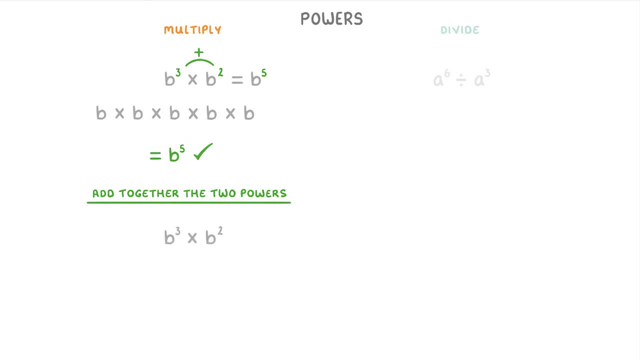 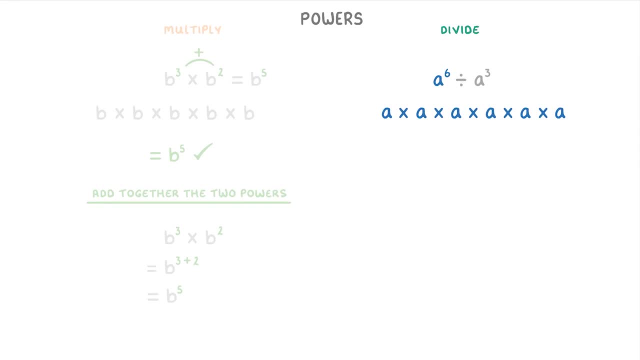 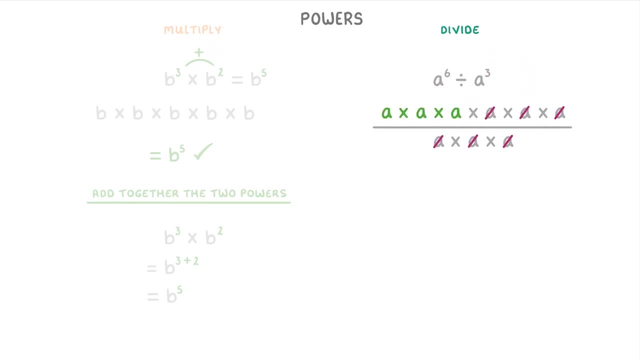 until we find that we'd only have three a's left on the top, And that tells us that our answer is a cubed Again, though there is a quicker way to do this, which, when we're dividing, is to subtract the two powers. So, for a to the power of six divided by a to the power of three, we just write: 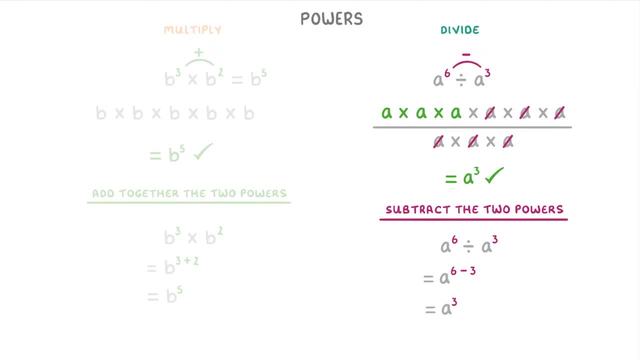 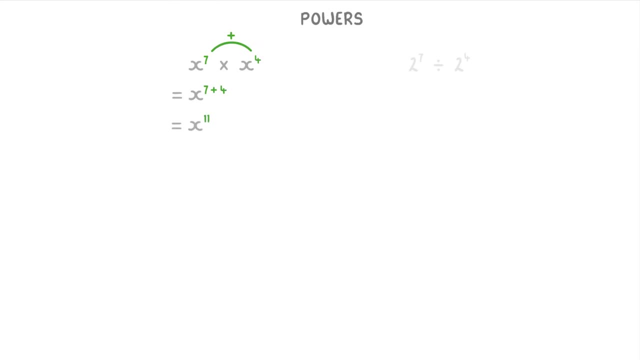 times a times 7 plus 4, which is x to the power of 11.. This next one, two to the power of seven, divided by two to the power of four, is a bit different because the base is a number rather than a letter, But it works in exactly the same way Because we're dividing. this time we have to 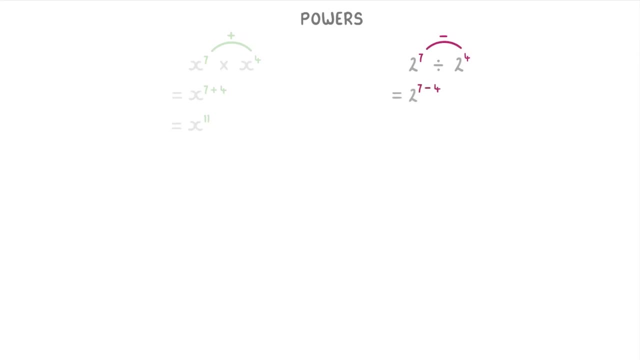 subtract the powers, So two to the power of seven minus four, which is two to the power of three. One extra thing we can do when the base is a number, though, is to work out its exact value, So because 2 to the power of 3 is just 2 times 2 times 2,. 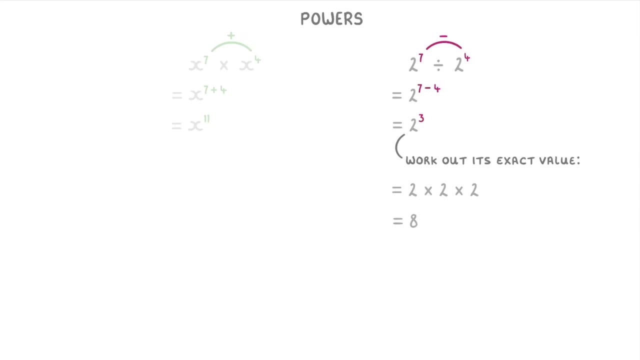 we can multiply them all together to find that the answer is 8.. For this next one, a to the power of 9 times a to the power of minus 5, we again just add the powers. So a to the power of 9 plus negative 5,. 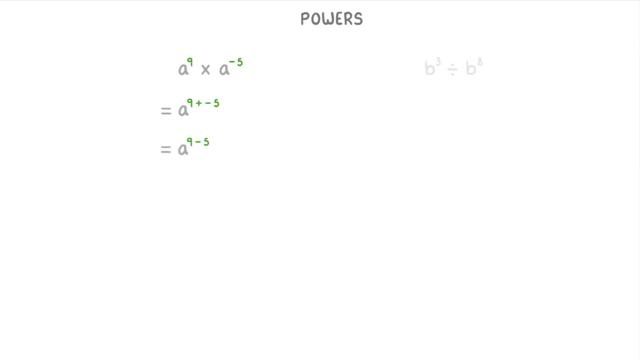 which is the same thing as a to the power of 9 minus 5.. So a to the power of 4.. Then for b cubed, divided by b to the power of 8, we just do b to the power of 3 minus 8,. 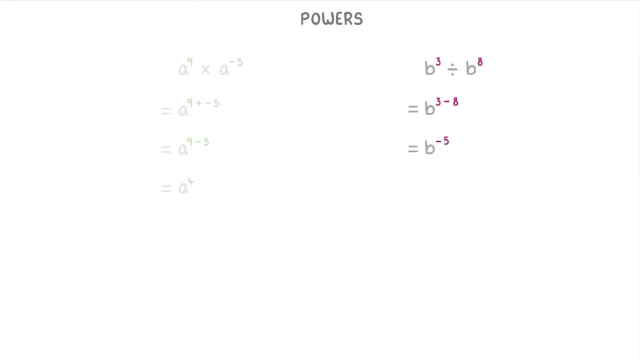 which is b to the power of negative 5.. And it doesn't matter that our power here is negative, That's absolutely fine. We can just add up all the powers. We don't have to do the same thing here. In this next one, we have three terms being multiplied together. 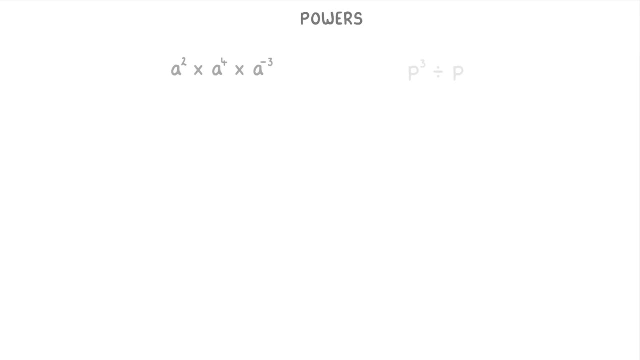 But the technique that we use is exactly the same. We just add together all of the powers, So a to the power of 2 plus 4 minus 3, which overall gives us a to the power of 3.. For p cubed divided by p, the p term looks like it doesn't have a power. 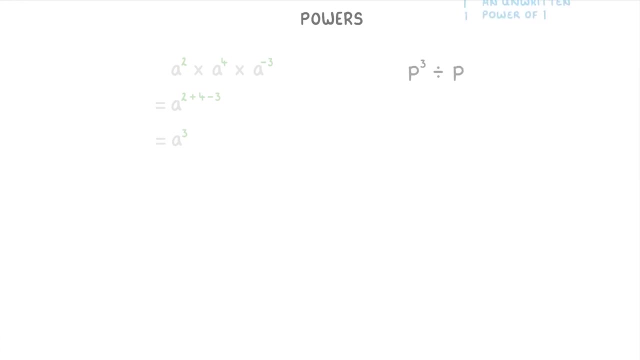 But whenever you have a number or letter, by itself it really just has an unwritten power of 1.. So we just do p to the power of 3 minus 1, which is p squared. One last thing to cover is that when you're doing questions like these: